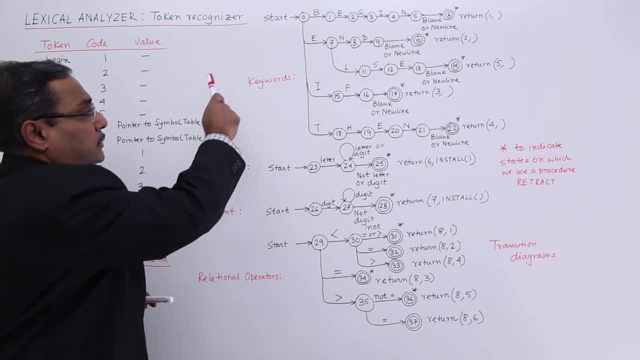 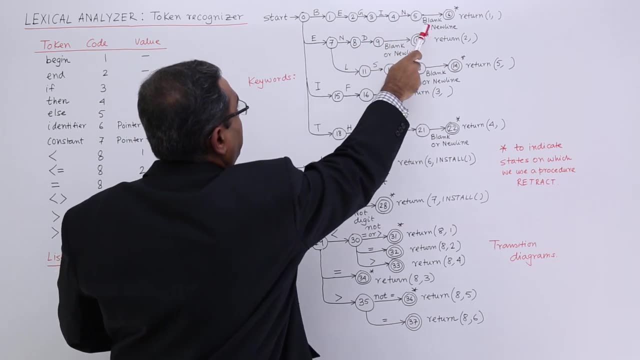 diagrams here: See so start. we have made this one deterministic, So now start state 0,, b, e, g, i, n, and after that if I get any blank or new line as a delimiter, then 6 will be the final state. 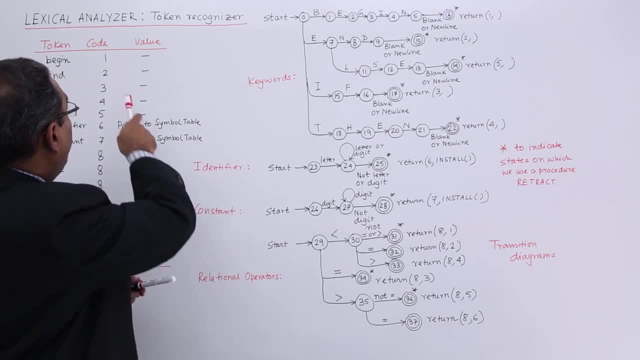 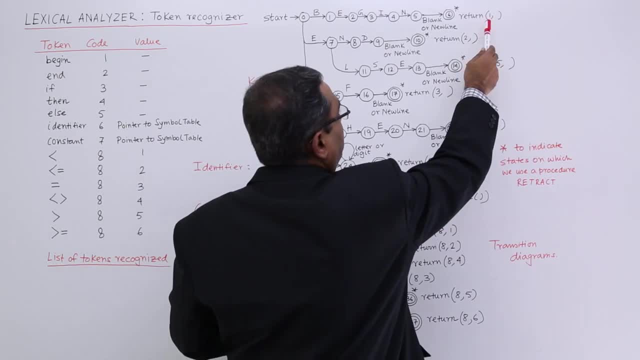 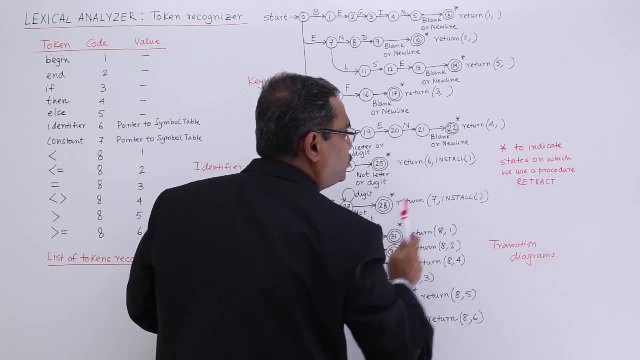 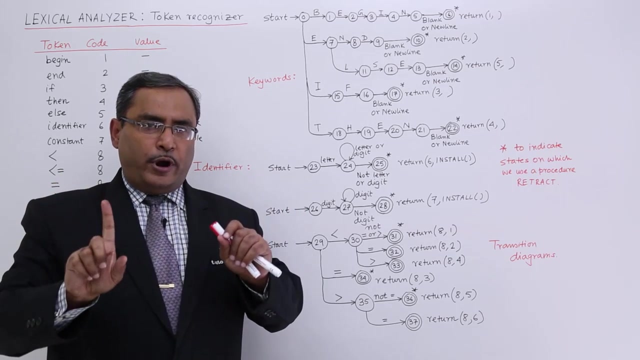 returning 1.. So that will be the code value. So return 1.. So it will be coming like this. Now, what about this? start Start to indicate states on which we use a procedure retract. In our earlier videos we have discussed that there will be one input buffer and the pointer. 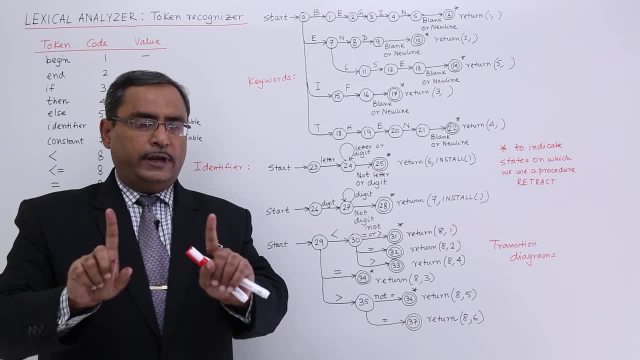 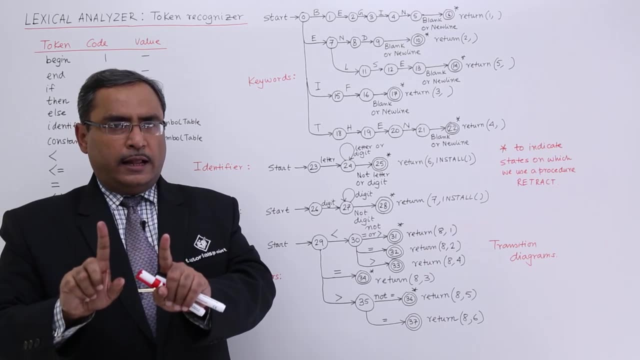 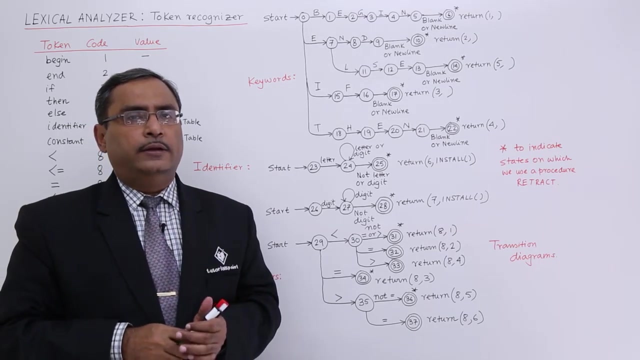 will be the token beginning pointer. Another pointer will be going in front and then in this case, in this case, what will happen? When it will get a delimiter, then it should retract and then, from this beginning of this token and this particular look ahead pointer, in between it will try to find 1 token. It. 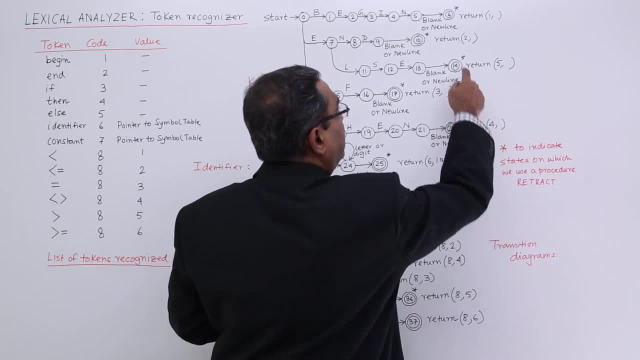 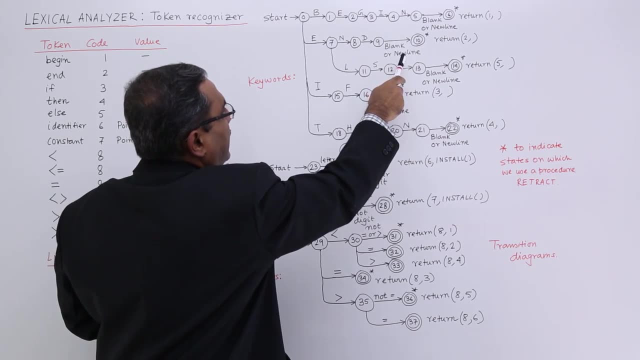 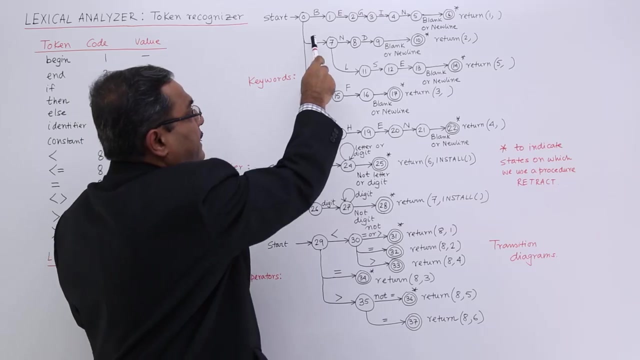 will try to analyze 1 token. So this start will indicate that in this particular state it must be doing the retract operation. E n, d, blank or new line as a delimiter start and then return 2 because the end will return the value code 2.. 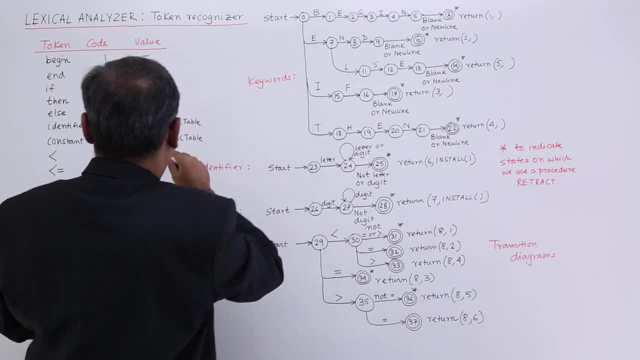 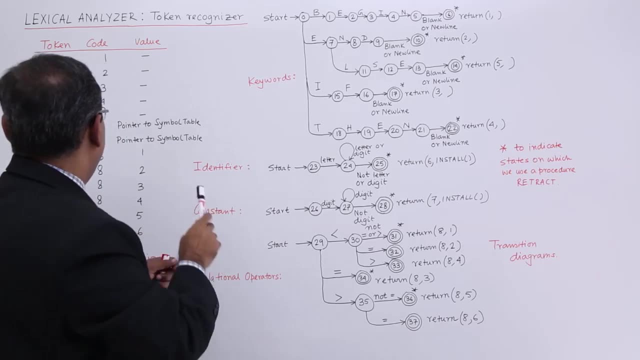 So 1, two, i m s, 1,, 2, p, l, a, s, e same thing. return 5 is the 5 as already a return, as else. So in this way, if you proceed, i f then blank on new line, return 3, because we will should. 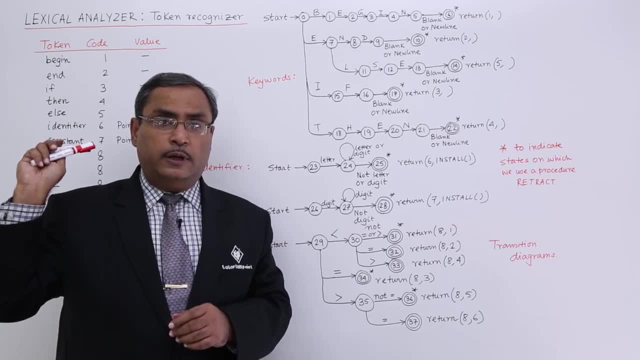 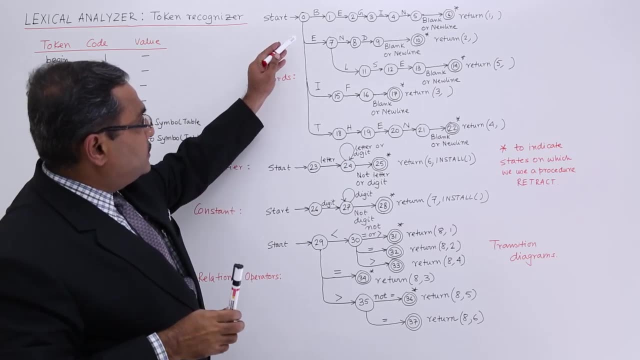 return 3 here. So accordingly, whatever the token recognizing the table is there. So we have to double up this transition accordingly. Now see from start t h e n. then blank our new line, Return 4, because then should be having value 4 here, So Number of the values. 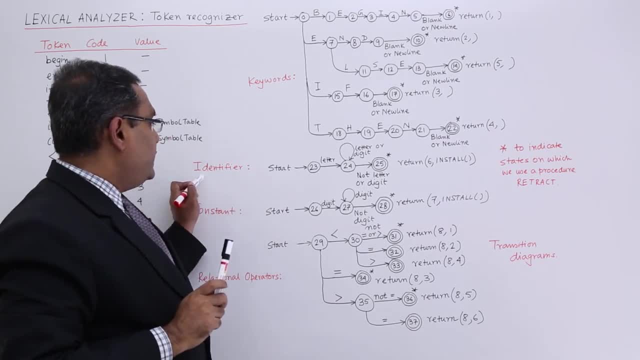 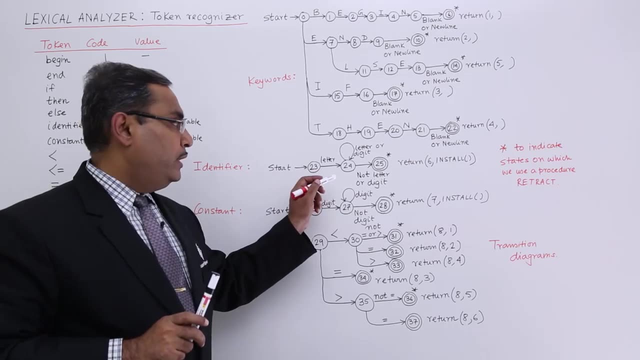 will getting 3.. So when this random angle, these two values are equal, one angle two, or having the value 4 here. So now for the identifier: start: letter, letter or digit. in our earlier video we have discussed this one in more elaborative way. So letter, letter. 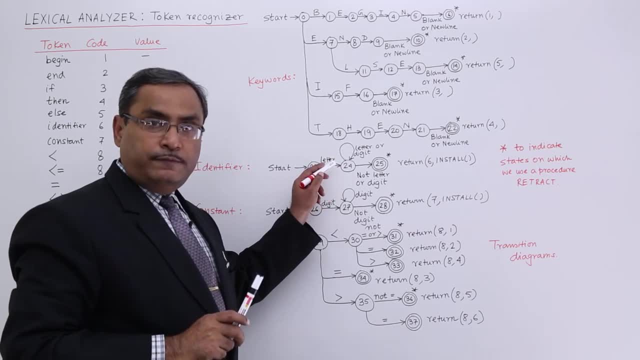 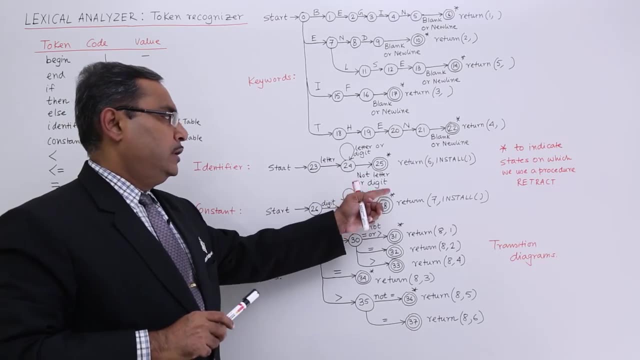 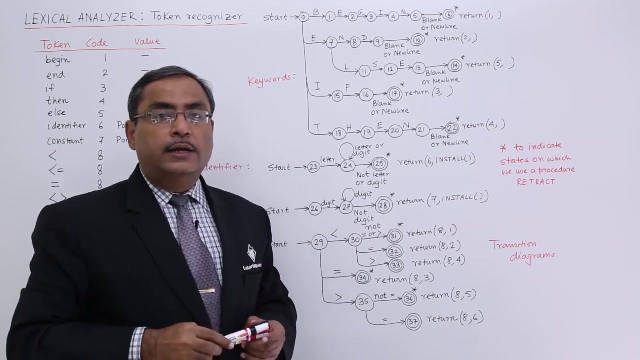 or digit, and so it will go for the state 24 is having a self loop and then not, not a letter, not a letter or not letter or digit, then it will go to 6 and install. So 6 and install will return. the install will write the symbol table. write this particular identifier in: 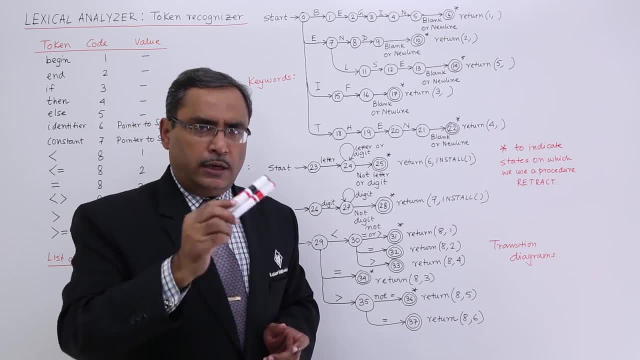 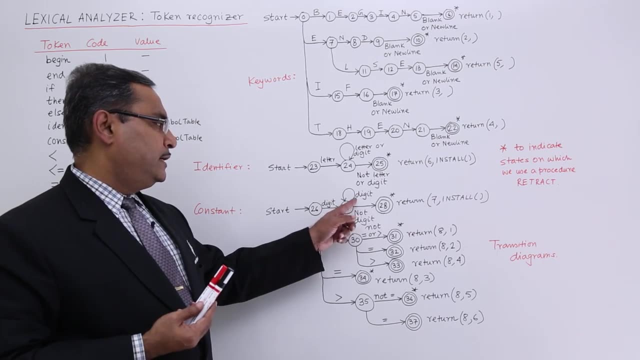 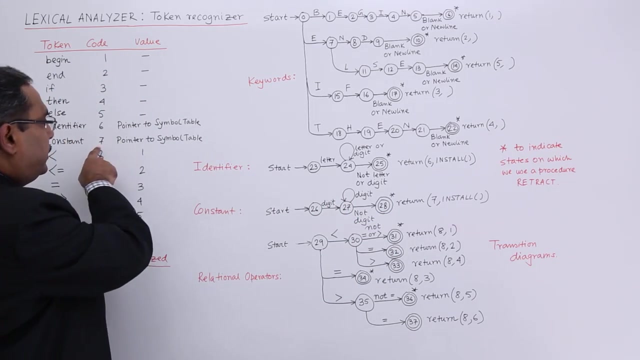 the symbol table and it it will return the address of that record entry. Now constant, digit. constant can be of single digit or multiple digits, So digit or digits. so self loop, not digit. So go for return 7 install. So accordingly it is working according. 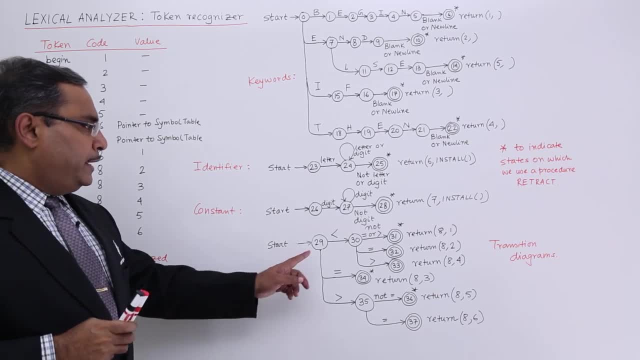 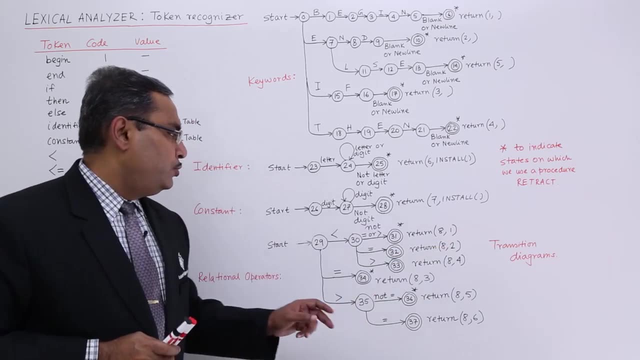 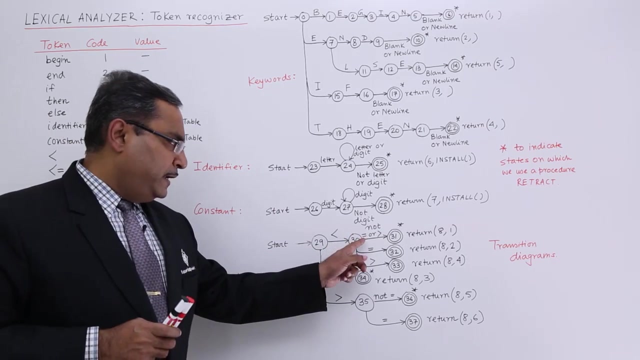 to this table. So now these are relational operators. we are having less than or less than equal to, So less than equal to 8, 2.. So return 8 2. it is not equal to return 8, 4, let me check- not equal to return 8, 4.. And if it is not equal to or not greater than, 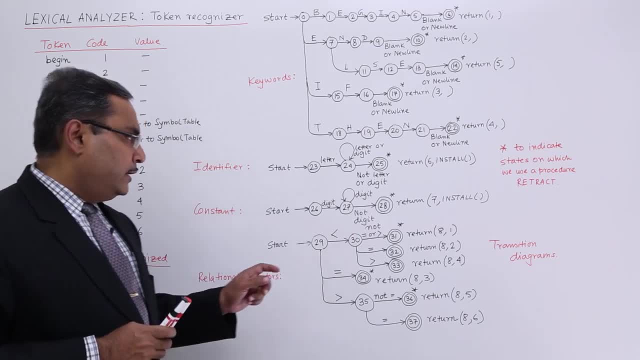 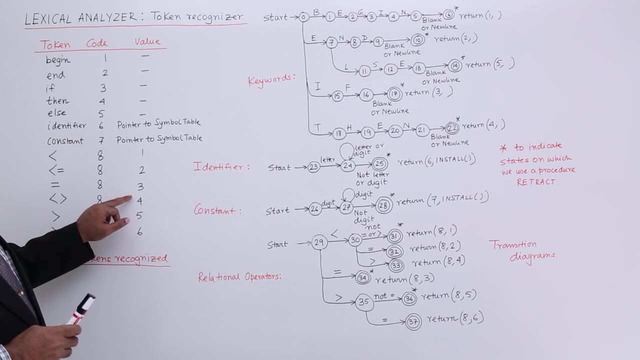 then it is only this, less than then: return 8: 1.. Similarly, only for equal to return 8: 3, only for equal to, it is 8: 3.. So, only for equal to, it is return 8, 3. 3. Now, greater than and greater than equal to, So greater than equal to return 8: 6, greater. 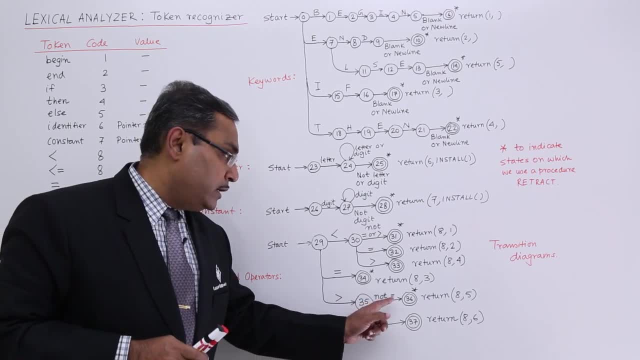 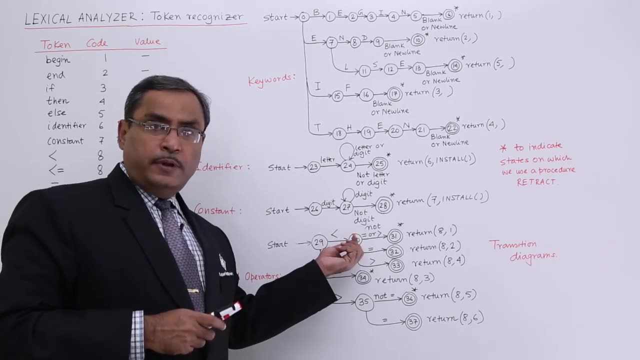 than, and it, if it is not equal to, then it will be treated as a delimiter, then this one. So in this way it will be working. So you see, not this, that means I have proceeded for one character. then I should come back. So retract will be required here. retract will. 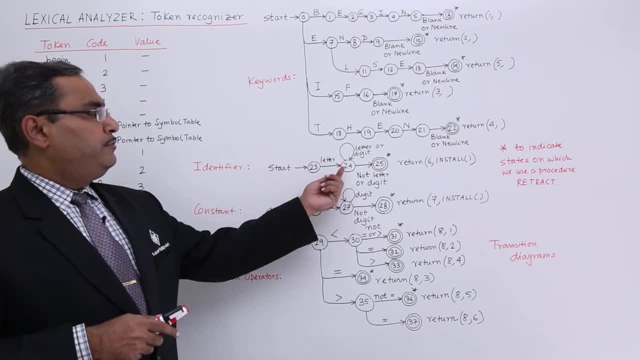 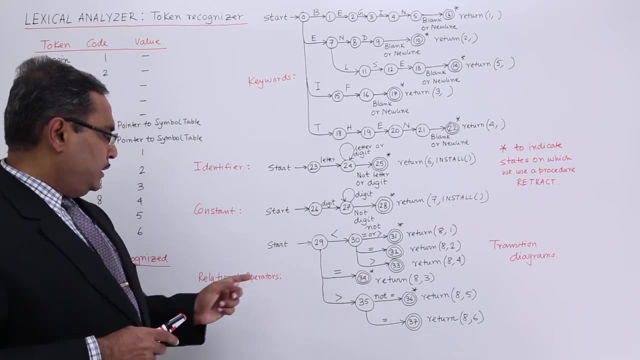 be required here. in this way, it is there working. ok, So retract will be. retract will be required here. retract will be required here. So star has been put in this way. you see relational operators. this is the constant. this is the transition diagram for constant transition. 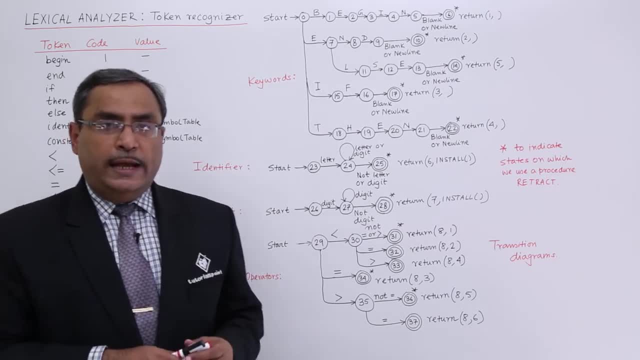 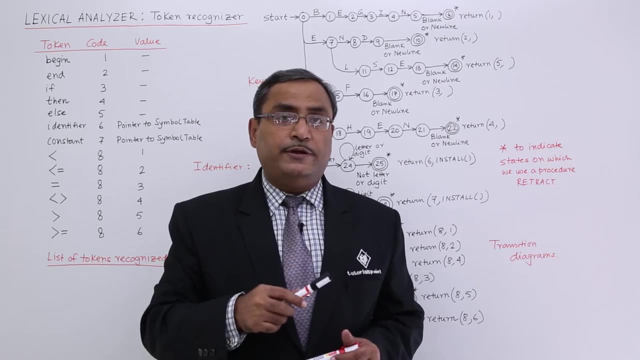 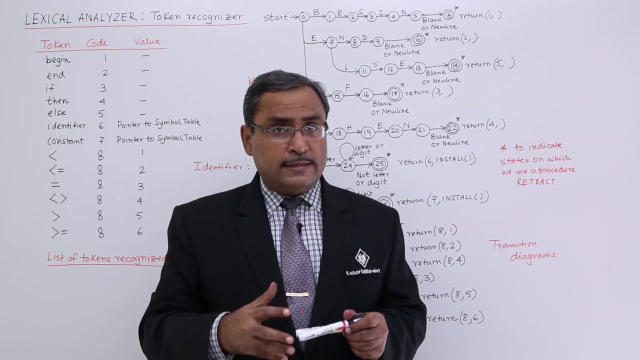 diagram for identifiers. transition diagram for the keywords. in this way is the list of token recognized and the respective transition diagrams. and you know, in our previous video we have shown you that from the transition diagram how to write the sample program code, So how this lexical analyzer will have the 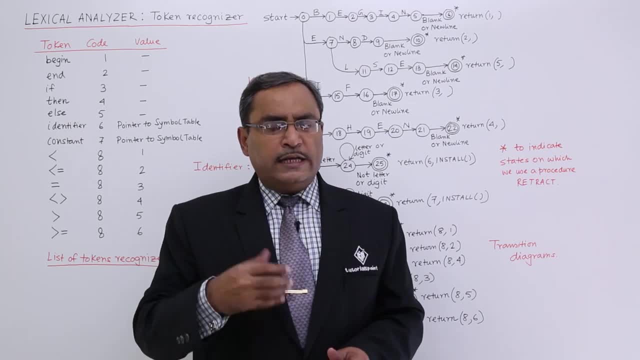 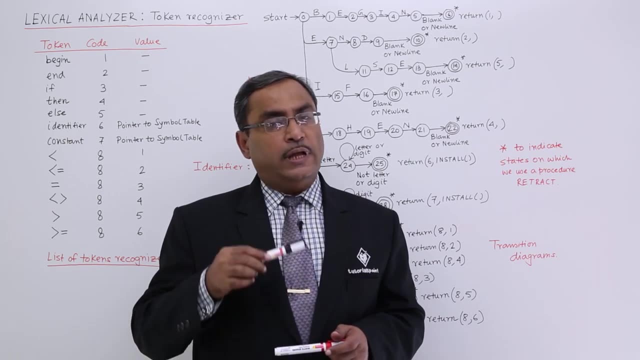 sample code. you are getting the idea, and in the next video we will be going for the lex program: how to write a lex program. what is the syntax, what are the sections? are there? So that video will be also in the continuation of this particular topic. please watch those videos. also thanks for watching this one.